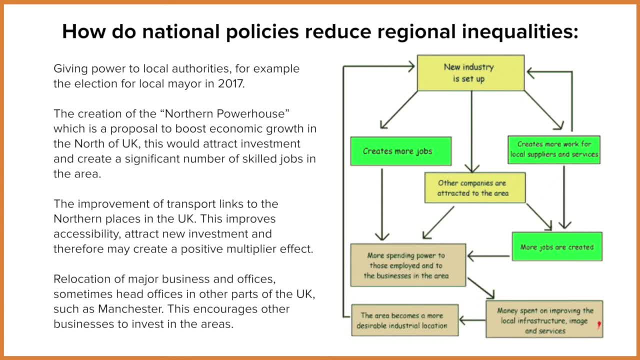 from tax to develop the infrastructure of the area, improve the image of the area and develop some more services like bus routes, And then that means that this area has become more desirable, both on an industrial level, to encourage more businesses to set up, but also. 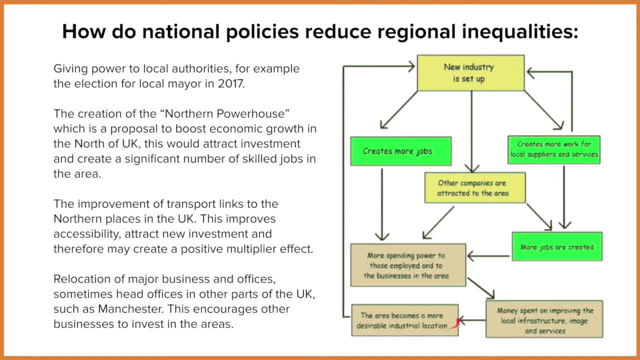 to maybe encourage more people to come and live in the area as well. So this has become a more desirable area, which then feeds back into well, it's starting up a new industry, which means more jobs, which means more spending power, which means improved services. So this cycle is going on and 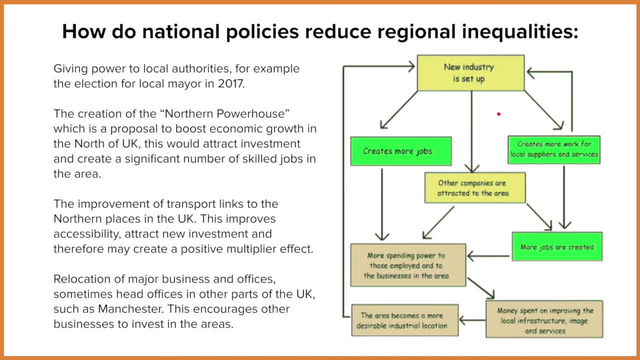 on and on. That's the theory. So let's have a look at it in one example. So if we use the North East of England, we're going to use Sunderland with Nissan. So Nissan set up in Washington, It created jobs for an area that was seen at high levels of unemployment because of the lack 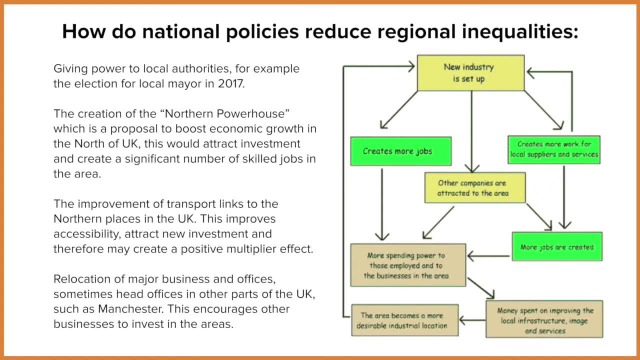 of available industry, because coal mining and shipbuilding had both declined over the last 20 years And the government encouraged Nissan to set up in that area. It created more jobs, which allowed the local economy to flourish because there was more spending power, But probably what's more important in terms of Nissan: Nissan builds cars. 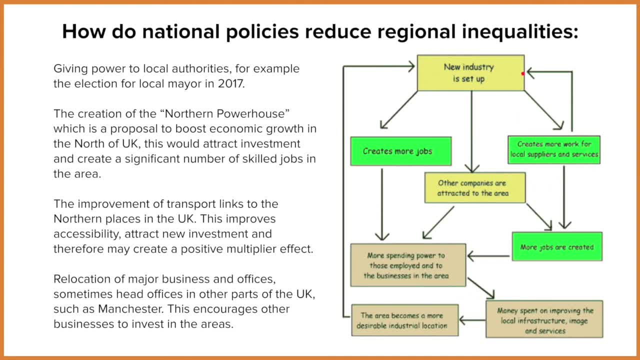 but it doesn't build all of the things that go into cars itself. So the manufacturing happens within the Nissan plant, but it needs additional things from the local area. So when Nissan set up, there were other companies that set up as well. So there were places that made tires, that made. 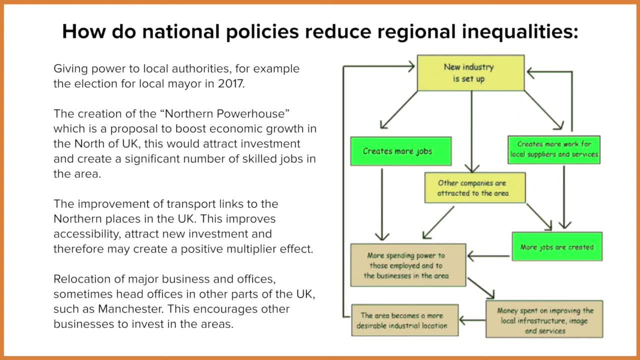 seatbelts that made the seats and the the carpets that went into cars. So when Nissan set up, it also encouraged lots of other smaller businesses that feed into Nissan to set up there as well, which also created new jobs, which also 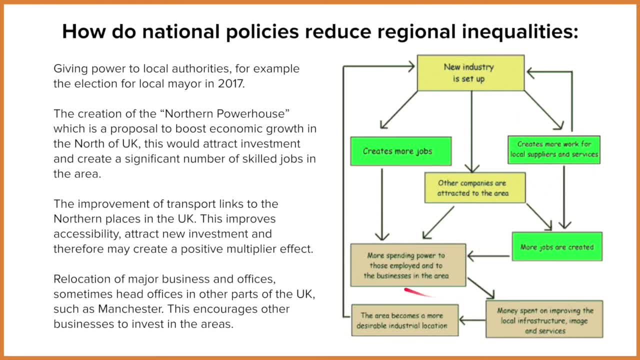 meant there was more spending going on. So you can see that this entire cycle is derived from one investment, which was the government encouraging Nissan to come to Sunderland and saying that they would get some tax relief and some additional support, But then that's allowed other businesses. 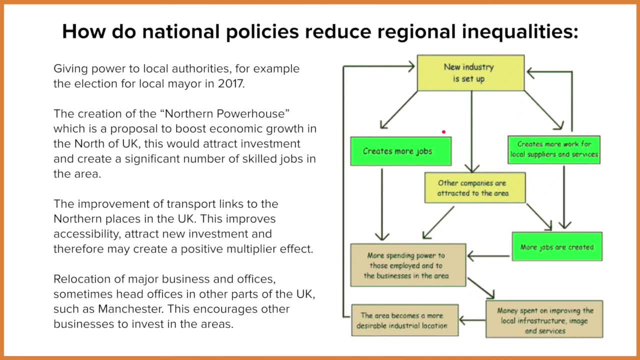 to set up and encourage this positive multiplier effect. to continue Some of the things that have happened nationally: Well, there's been the Northern Powerhouse scheme, which was a proposal to boost economic development in deprived areas of the North. So the idea was that this was a national campaign to drive investment into the North and also move some of 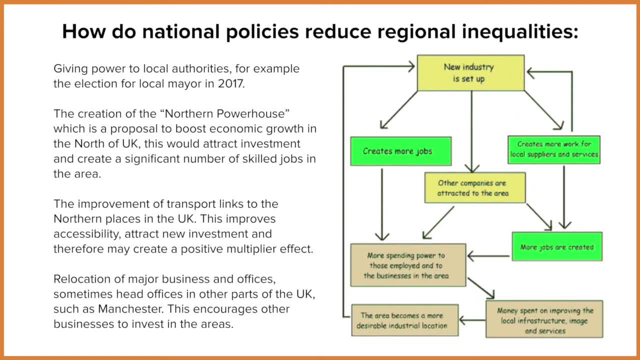 the key government services further North as well. So instead of basing them all in London, they'll be moved further North. Part of the Northern Powerhouse was allowing for improved transport, So you might have heard of HS2,, so High Speed Railway 2.. And while it doesn't come all the way up to the North East of England, it does. 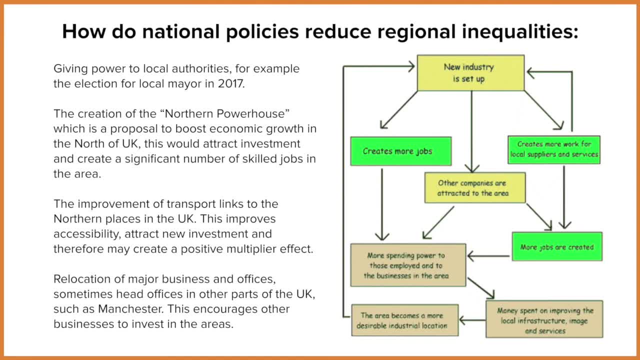 go into the North. So the idea is that an increased amount of mobility to places like Manchester Leeds area would mean that it would encourage more businesses to perhaps set up further North because they could commute easier with London but also allow more people to commute further South as well. And then the idea of trying to encourage more businesses. 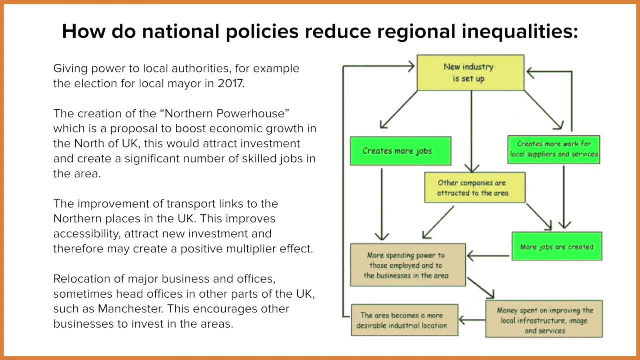 and offices to move their headquarters, their HQ's, further North as well. We've seen this probably the most with technology and media. So the BBC, Channel 4, have both moved their broadcasting centres to the further north. so the bbc's moved theirs to media city in manchester and salford. so this is 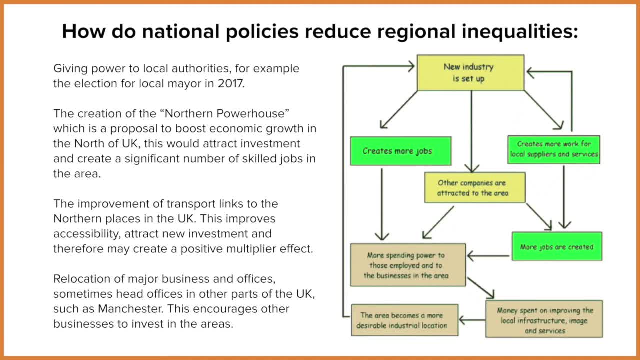 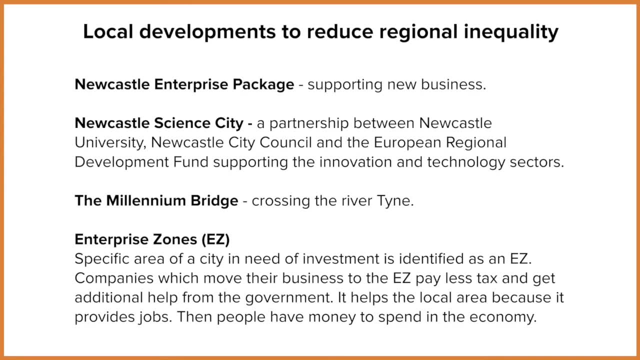 encouraging more investment further north, where they've always been traditionally centered in the capital, in london. if we look at something a bit more local to us, there's been a couple of different strategies that have been attempted. so there's the newcastle enterprise package. so this was 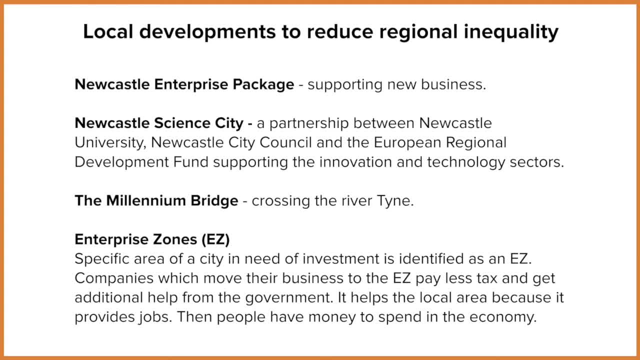 governmental and local government support for businesses, so providing cash incentives and tax relief to encourage more businesses to set up. there's the newcastle science air city, which was a partnership between a couple of different institutions, so there's newcastle university. there was the eu with their regional development fund providing some money, and there was some